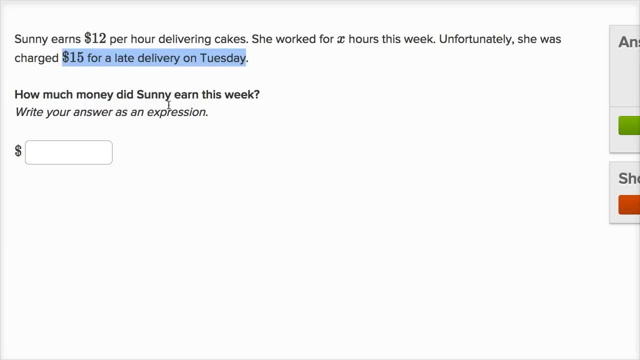 for her late delivery on Tuesday. How much money did Sunny earn this week? So if you see that she earns $12 per hour and she worked for x hours, say okay, she got $12 per hour. times x hours, So that's how much she would have made. 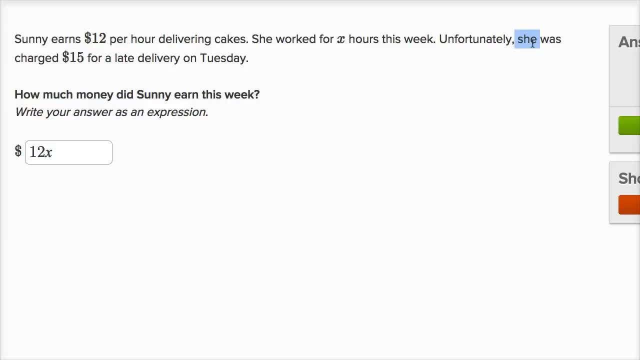 except for the fact that she also had. she was charged. I guess her employer charges her for late delivery, so she had to take $15 out of her paycheck. So this is what she would have gotten paid, based on her hourly wage and the number of hours she worked. 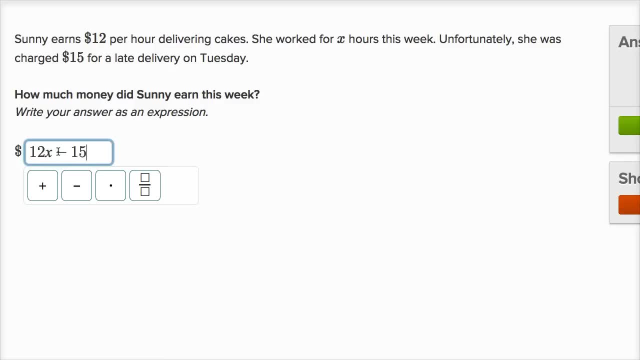 but then she has that late fee that she has to pay. So it's gonna be 12x minus 15 is how much she actually earned this week. Let's do a few more of these. There are C players on the Cougars hockey team. 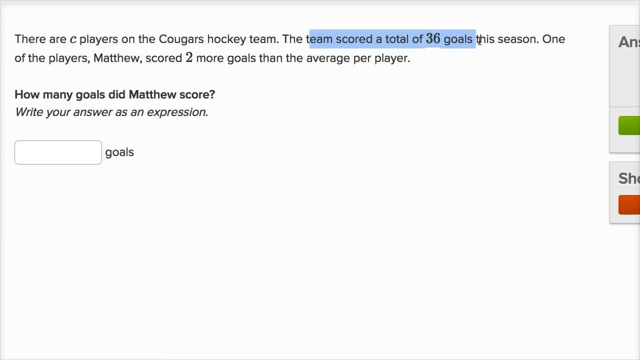 There are C players on the Cougars hockey team. The team scored a total of 36 goals this season. One of the players, Matthew, scored two more goals than the average per player. How many goals did Matthew score? All right, well, let's think about the average per player. 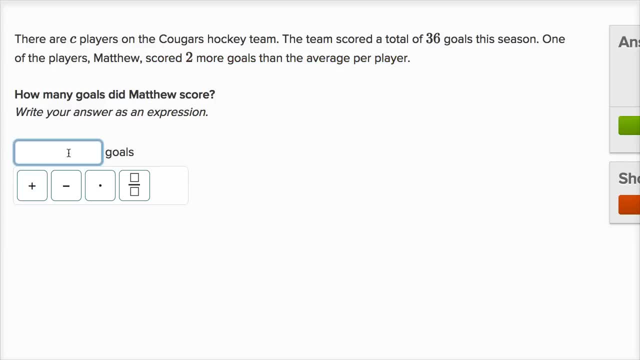 because we know he scored two more than the average per player. So the average is going to be the total number of goals divided by the number of players, and they tell us that they're C players. So this expression right over here, that would tell us the average. 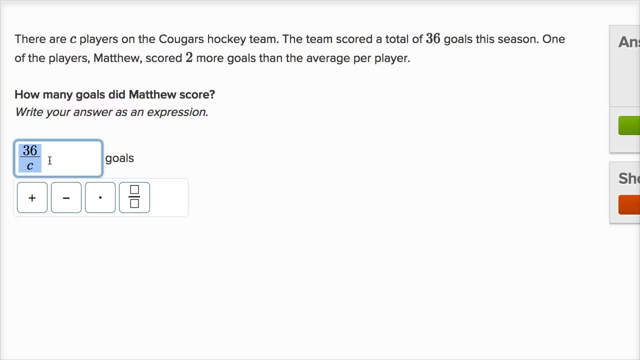 that's the average goals per player. Now we know Matthew scored two more than this thing over here, so we can just add two to that. and that's how many goals Matthew scores. Let's check our answer And the key here. this might seem a little confusing. 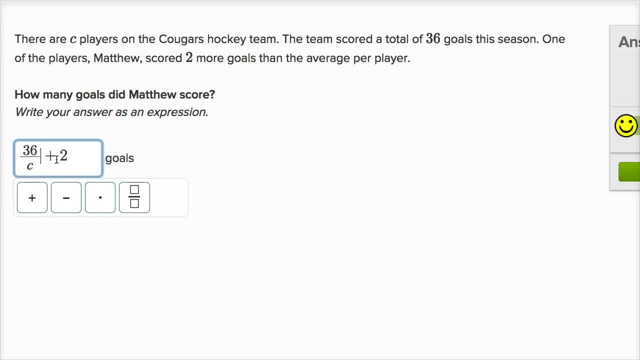 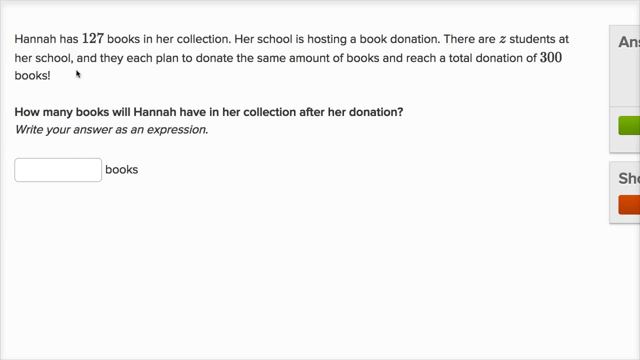 but remember: this says: Matthew scored two more goals, two more goals than the average player. The average player, the average goals per player, is 36 divided by C, is 36 divided by C. Let's do one more of these. Hannah has 127 books in her collection. 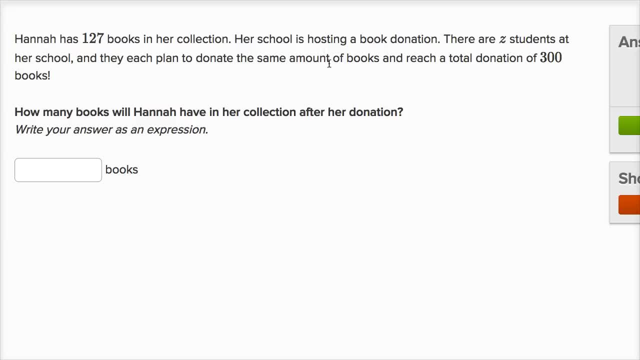 Her school is hosting a book donation. There are Z students at her school and they each plan to donate the same amount of books and reach a total donation of 300 books. How many books will Hannah have in her collection after her donation? All right, so let's think about it.